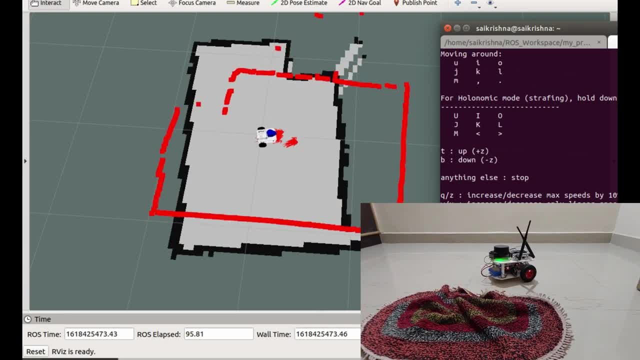 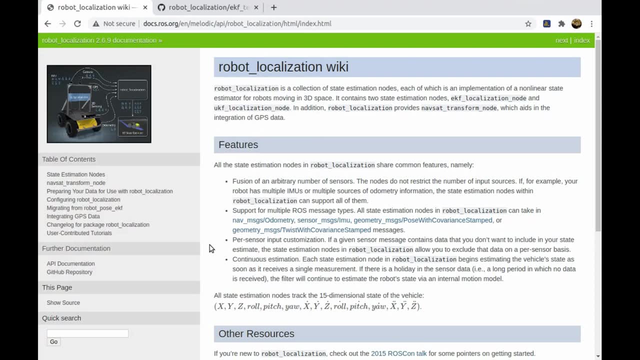 So, due to this mismatch in odometry data and the real state of the robot, AMCL node fails to localize the robot in the map. To improve this condition, we have to make the odometry data more reliable to match with the real state of the robot. 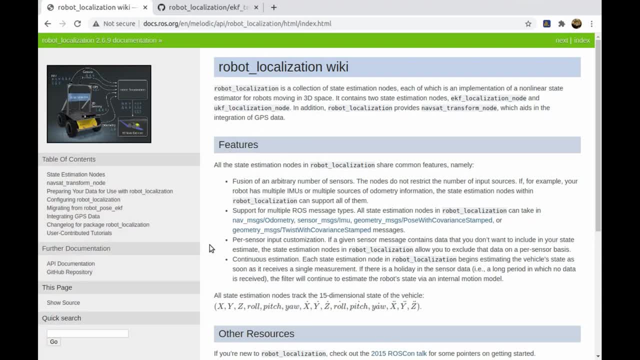 We can do this by sensor fusion. We can add another sensor like IMU, which can track the rotations and accelerations of the robot and fuse the IMU data with wheel odometry to get more accurate robot odometry. For sensor fusion in mobile robots we can use Robot Localization. 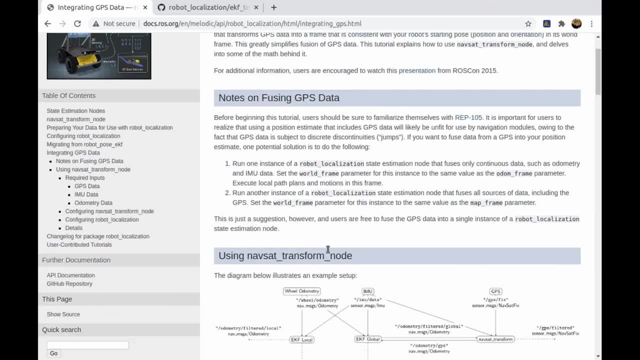 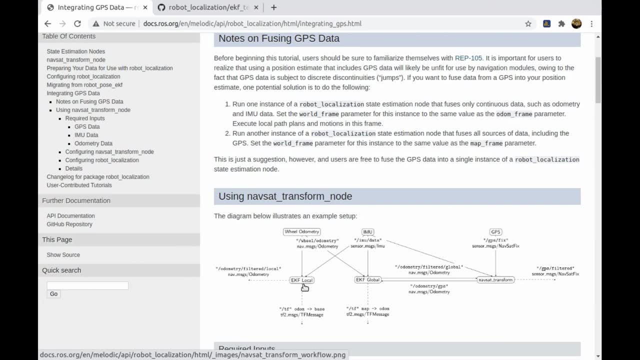 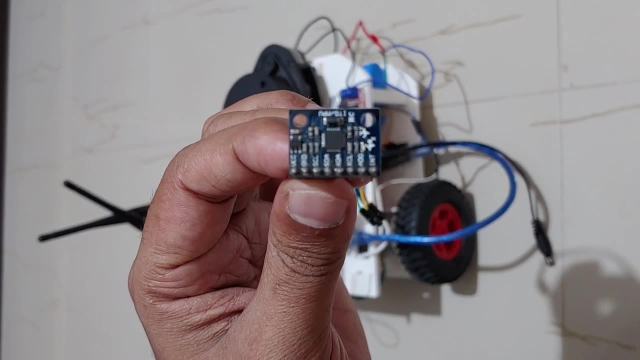 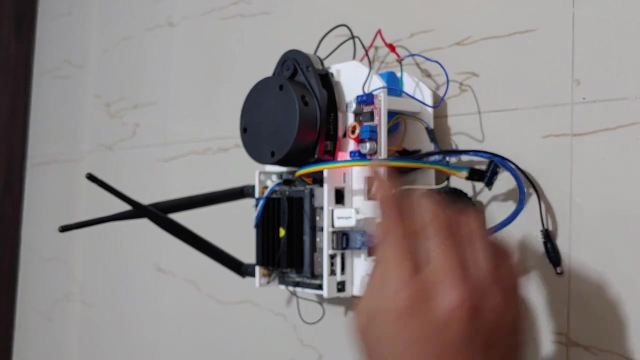 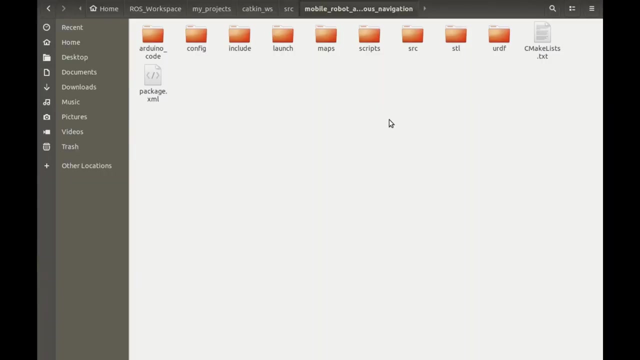 package. This package can be used to fuse wheel odometry, IMU sensor data and also GPS data. It internally uses Karlmann filter to predict the real state of the robot. robot with the fused data, I am adding MPU6050 IMU sensor to my robot. 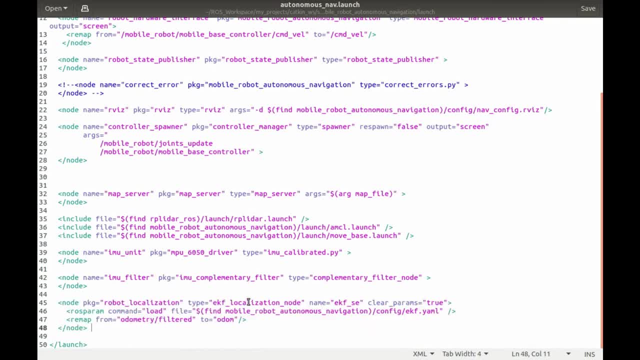 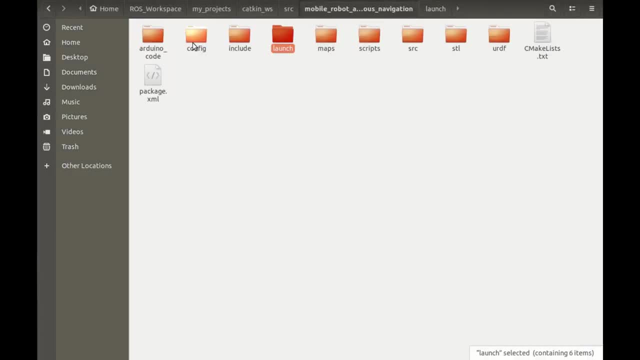 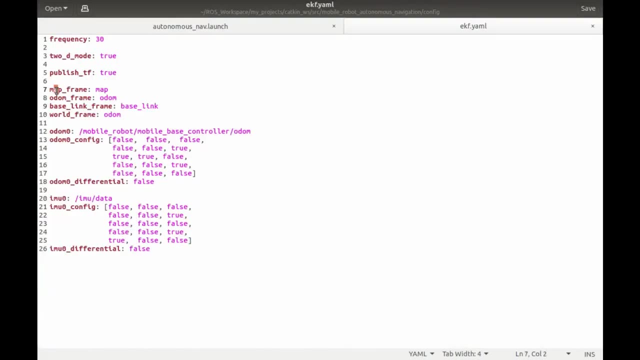 To use robot localization package. all we have to do is just add this node in the launch file and setup its parameters. Let's have a look into the parameter file. This file contains information of frame IDs, input sources, ie real odometry data- and. 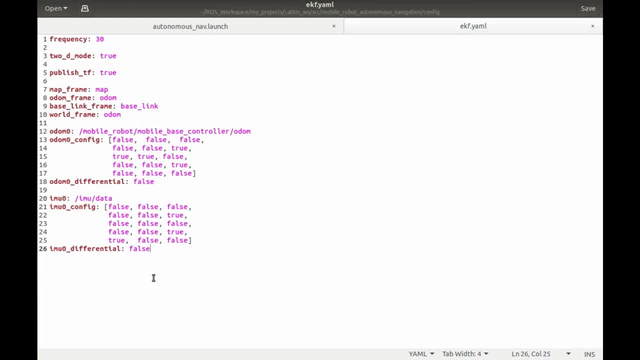 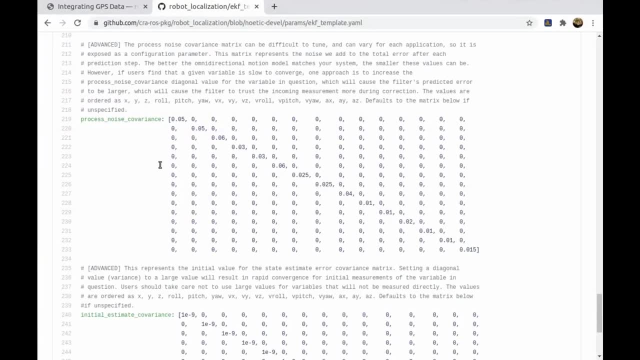 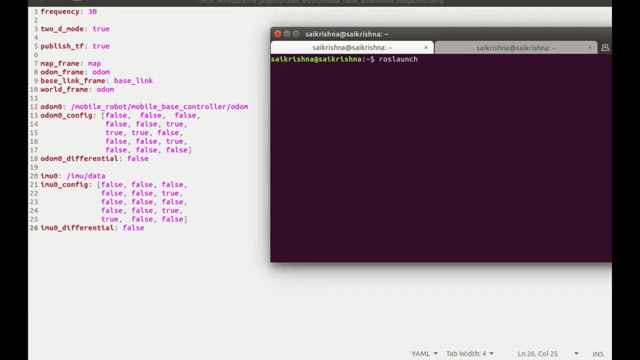 IMU sensor data. Also, we can add covariance matrices for Kalman filter. As I did not write any covariance matrices here, the default values will be used. These are the default covariance matrices. Now let's launch this file and test the robot's localization by driving over the. 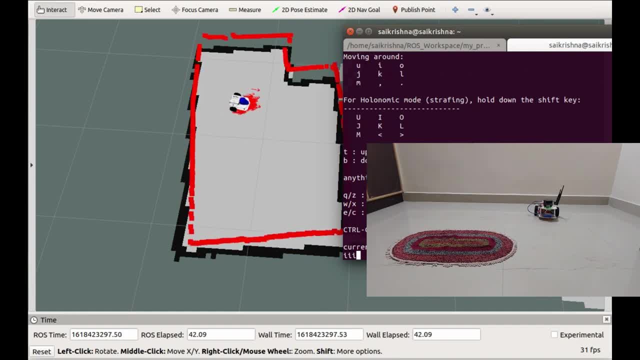 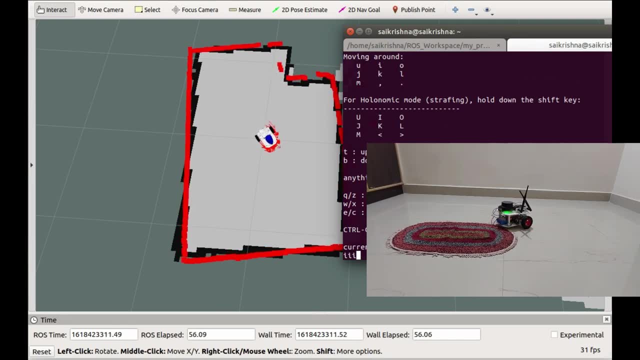 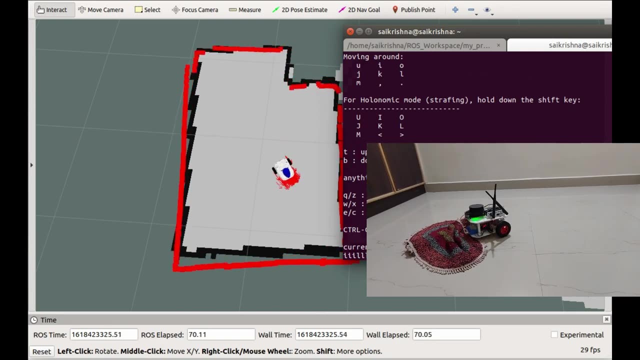 360 degree circular path, Even though we drive the robot on bat surface. robot's location in the map is proper. You know that I have set up the location as correct, which is fine. We will now see how it works in real-time. The first step is to add the robot's location.